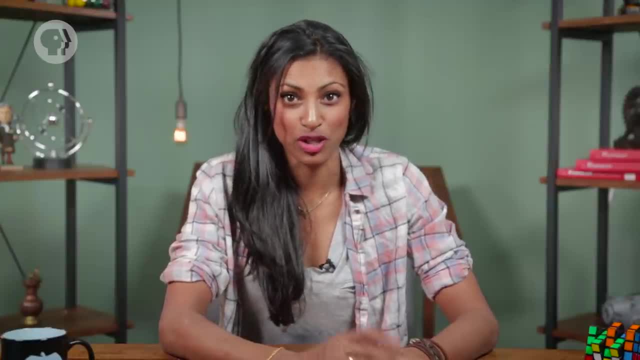 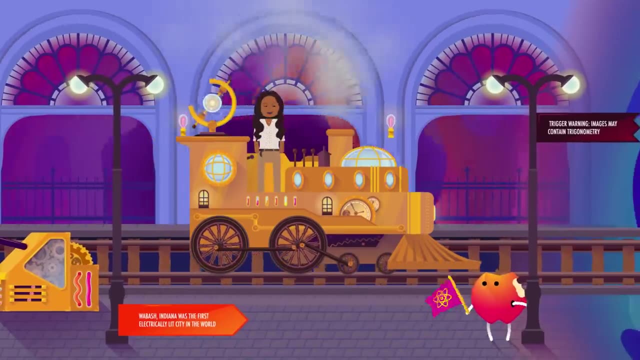 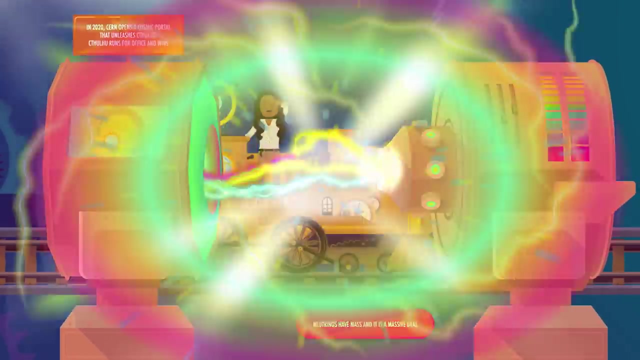 But it also makes doing other things pretty hard. Anyone who's moved furniture knows that. Luckily, friction is also a force, so as physicists, we know what to do with it. You're moving into a new house and you ask a friend to come help out, Which he does. 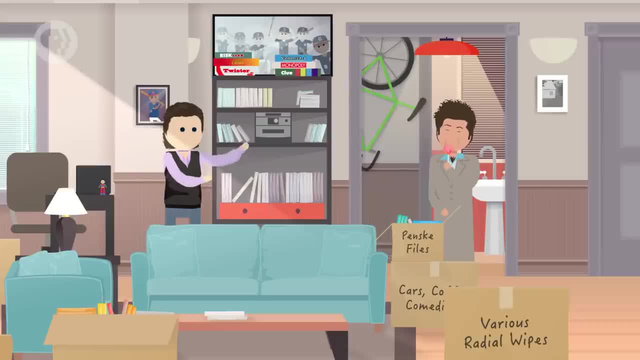 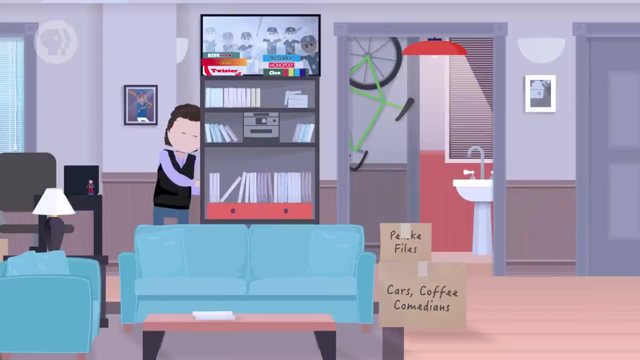 because he's just nice like that And you really do need his help because you have to move giant bookcases and a desk and you can't do it alone And about halfway through the move-in you're rearranging the furniture in your new bedroom. 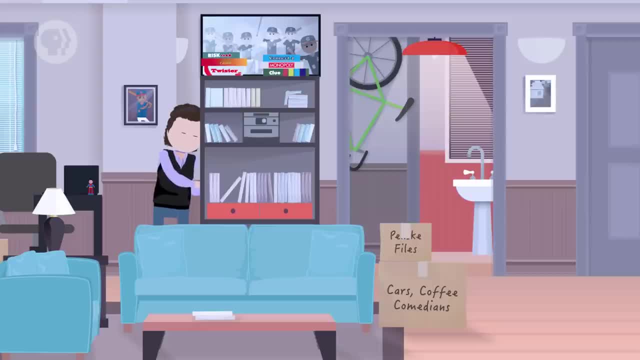 when you run into a problem. You're pushing and pushing on your bookcase, but it's just not sliding across the floor. So you call your friend over from the other room and, with both of you pushing, the bookcase finally starts to slide. 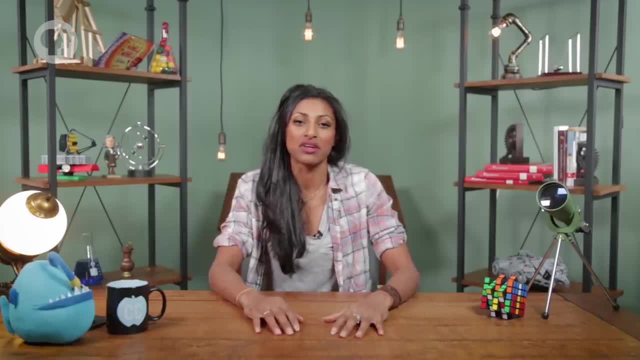 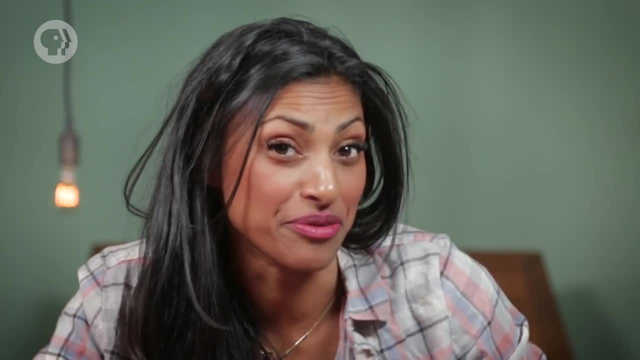 But it was really hard to get it moving and stay moving because there's a force working against you stopping the bookcase from sliding: Friction. And there are actually two kinds of friction. First there's kinetic friction – that's the force that slows the bookcase down as it slides. 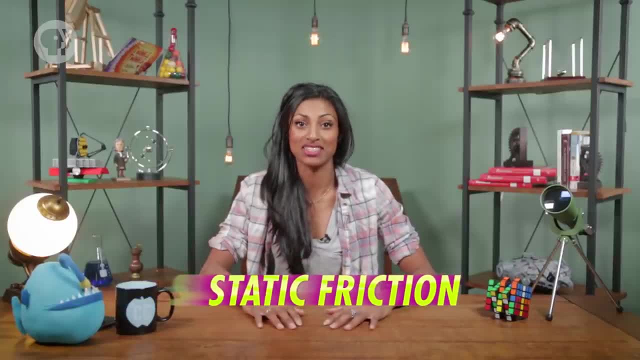 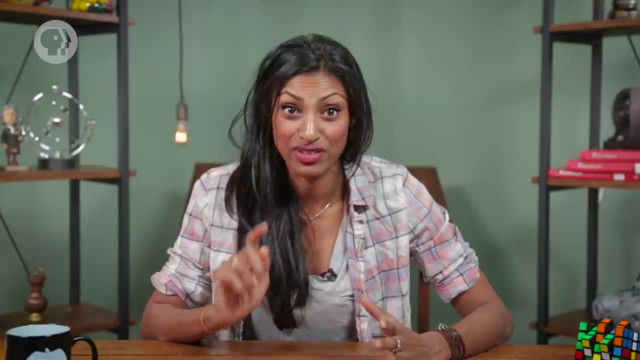 And then there's also static friction – the force that you had to overcome to get it moving in the first place. So let's talk about kinetic friction first. It's a resistive force, which just means that no matter what, it'll act to resist you. 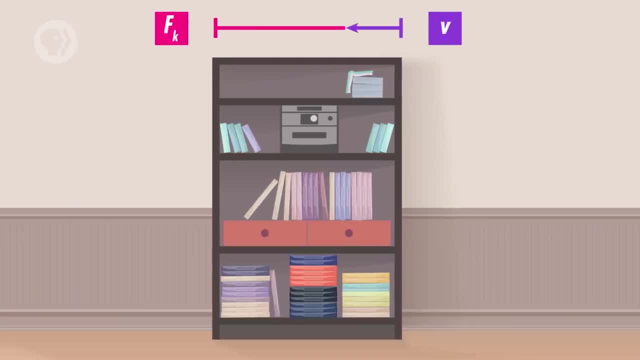 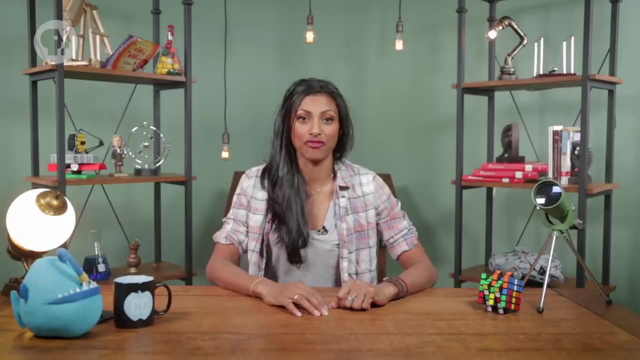 In other words, if you push the bookcase so it slides to the left, then the force of kinetic friction is acting to the right, But if you move the bookcase to the right, then the friction will resist to the left. Kinetic friction will also often generate heat or sound or both. 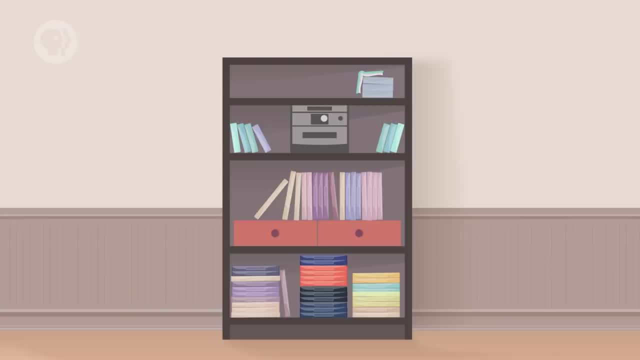 So what causes it? The bookcase and the wood floor might look smooth, but if you looked at their surfaces under a microscope, you'd see that they're covered in tiny bumps and grooves. As the bookcase slides across the floor, the surfaces catch on each other and might even 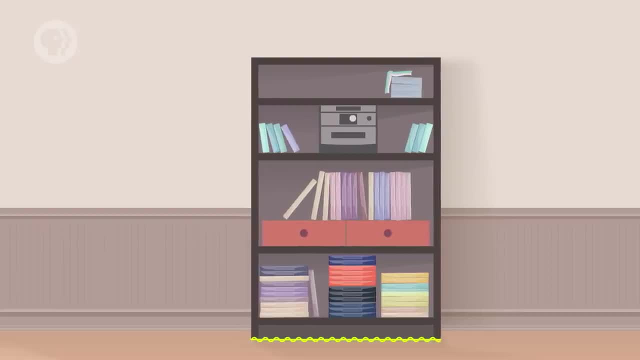 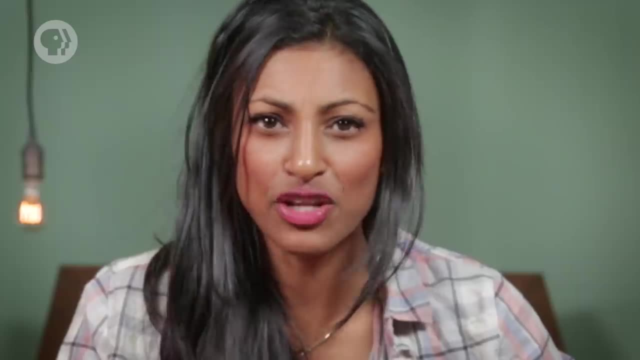 start to form weak intermolecular bonds. That pulls on the bookcase, slowing it down. But as the bookcase continues to slide, it breaks those bonds and moves past whatever bumps it was stuck on. The newly freed molecules start to spring back and the movement produces heat and sound. 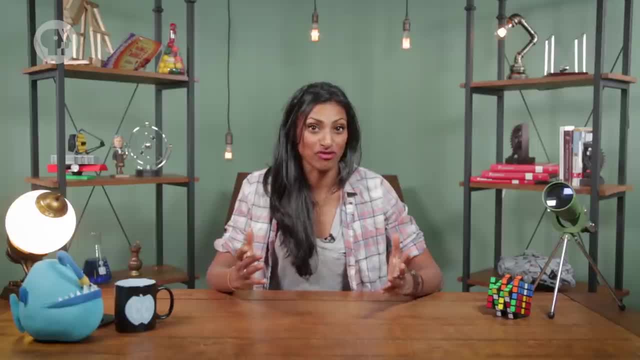 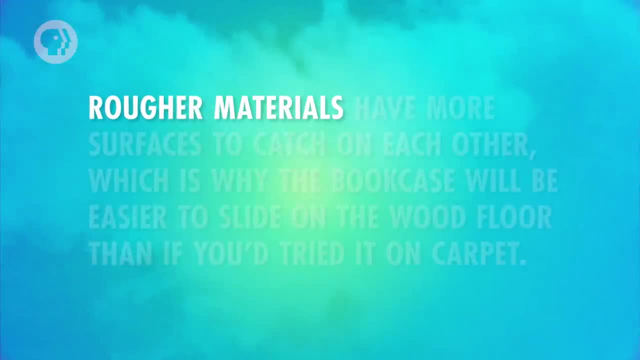 Then the cycle continues with the next patch of floor. You end up with a force that resists any kind of sliding movement, and its strength depends partly on what materials are sliding against each other. Rougher materials have more surfaces to catch on each other, which is why the bookcase will. 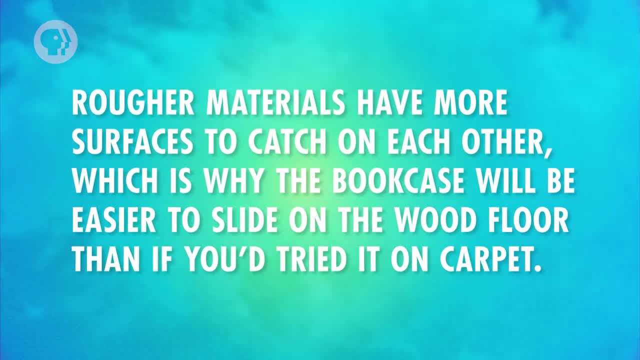 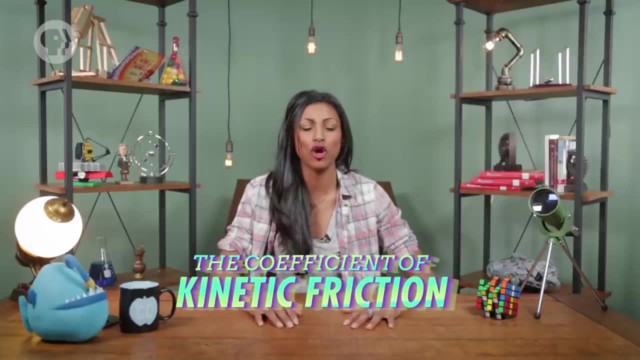 be easier to slide on the wood floor than if you tried it on carpet, And the way in which this roughness affects kinetic friction is called the coefficient of kinetic friction and it's different for pretty much every combination of materials. But there's another factor at work in friction: How hard the materials are pressed together. 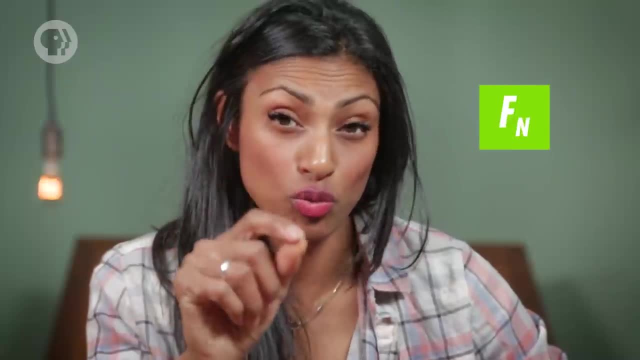 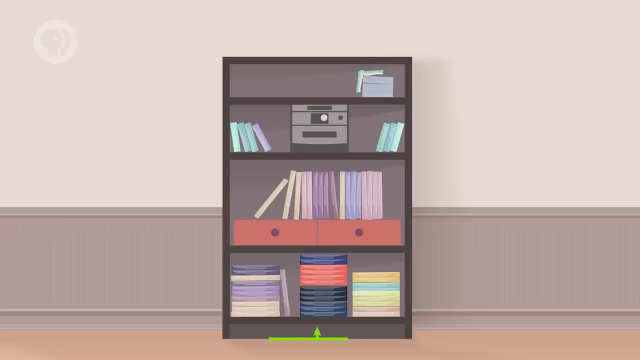 puts more of their surfaces in contact with the material, And that's where the normal force, or Fn, comes in. You might remember from our last episode that when a force pushes on a bookcase against the floor, the floor pushes right back. That's Newton's third law and we call the force. 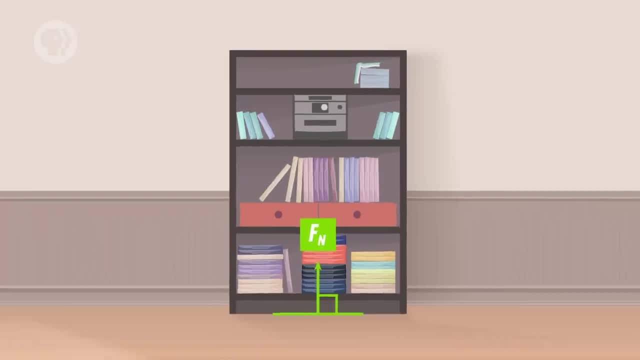 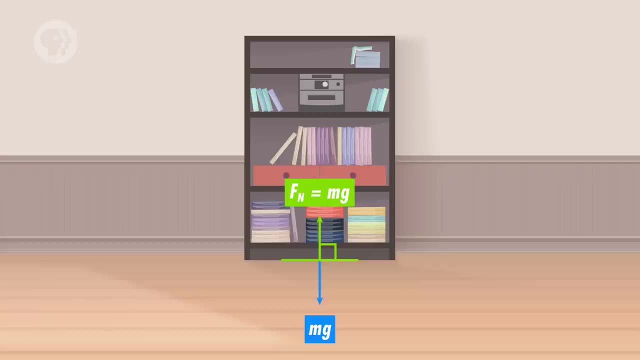 from the floor on the bookcase. the normal force, In this case the force from the bookcase on the floor, is just its weight, mg. So the normal force would be equal to mg, but pointing up equal and opposite. So now we know about the two main factors that affect the strength of kinetic friction. 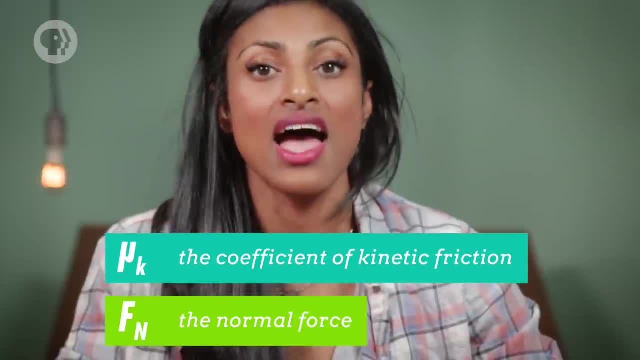 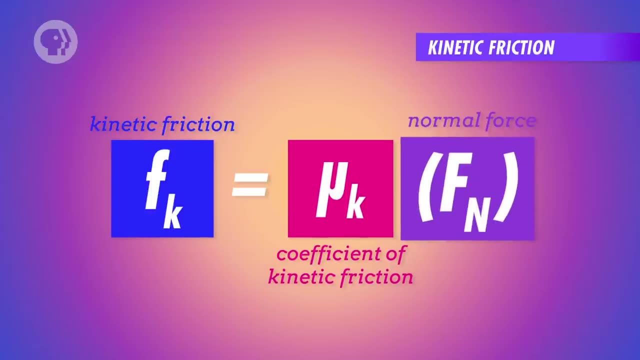 The coefficient of kinetic friction, written as muk, and the normal force Fn. It shouldn't be too surprising, though, that the equation for kinetic friction is just the coefficient times the normal force, But that's only half the picture. What about static friction? 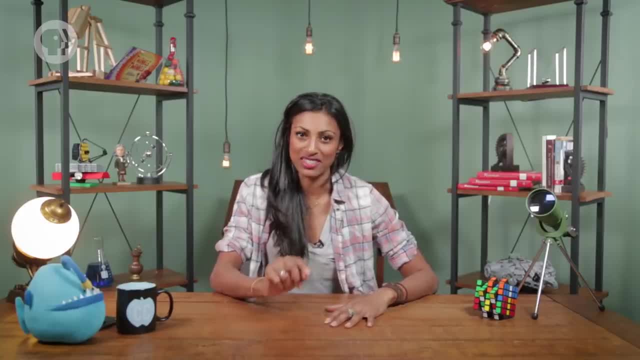 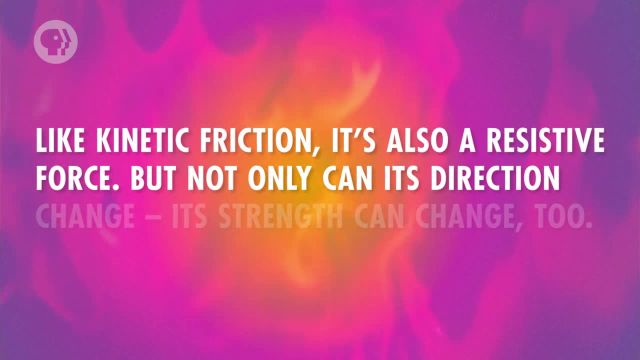 When you weren't able to move the bookcase to begin with, that was because of the static friction between the bookcase and the floor. Like kinetic friction, it's also a resistive force, But not only can its direction change, its strength can change too. 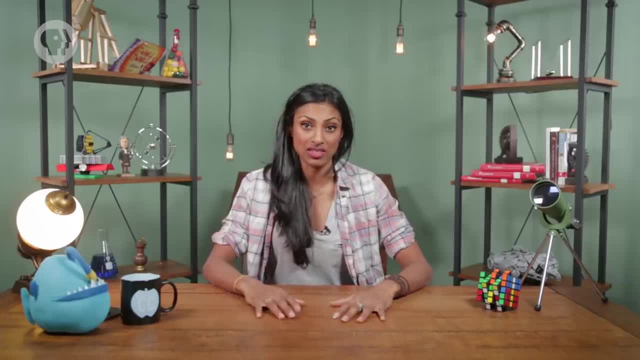 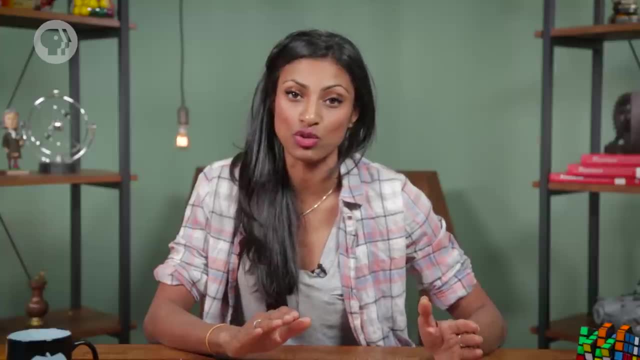 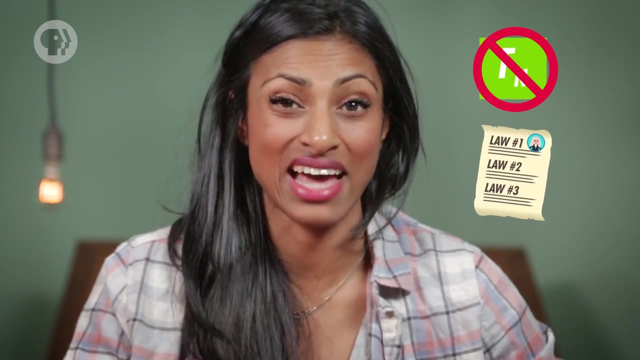 The bookcase must be in equilibrium, meaning that the forces on it balance out. So the force from static friction must be exactly equal to the force from your hand, but in the opposite direction. because of that equilibrium It's not the same as the normal force and it has nothing to do with Newton's. third: 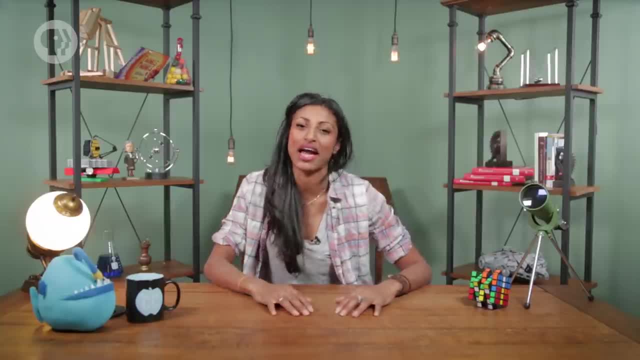 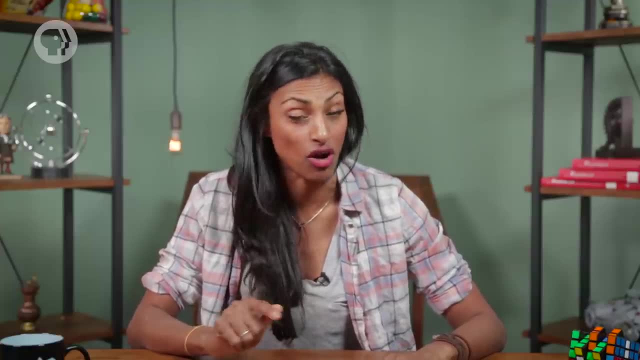 law, But say you really put your back into it, pushing as hard as you can. The bookcase still doesn't move, so static friction must still be pushing back with the same amount of force you are. However, the static friction between two objects can change Once your friend starts pushing. 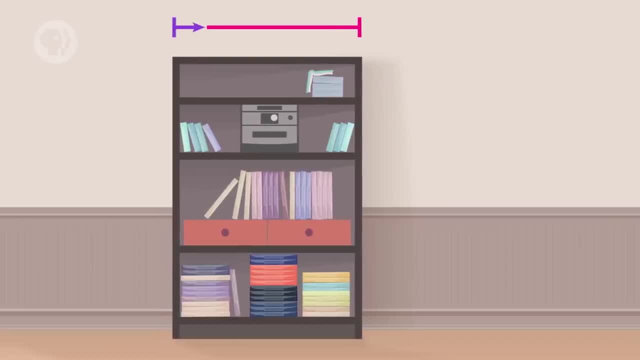 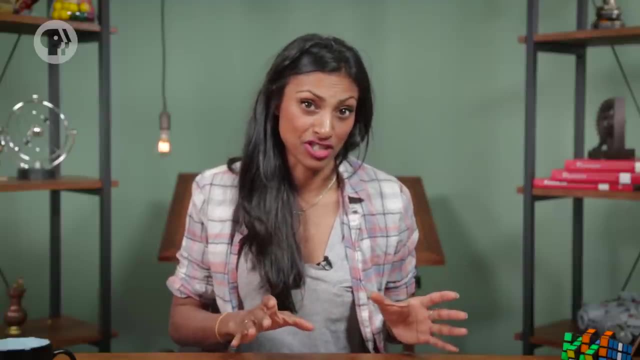 too, the bookcase starts to slide, because the force from your teamwork is greater than the maximum amount of static friction, which we write like this, And the relationship between the maximum static friction and the normal force is similar to the relationship between kinetic friction and the normal force. 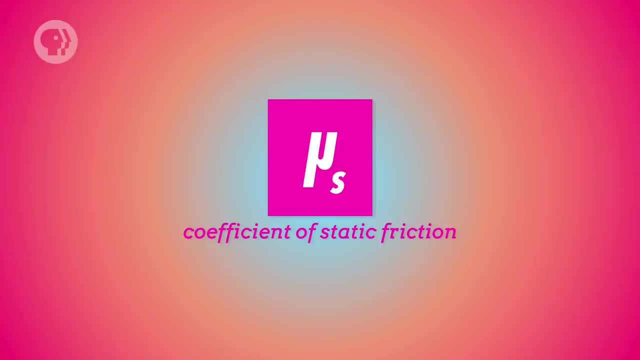 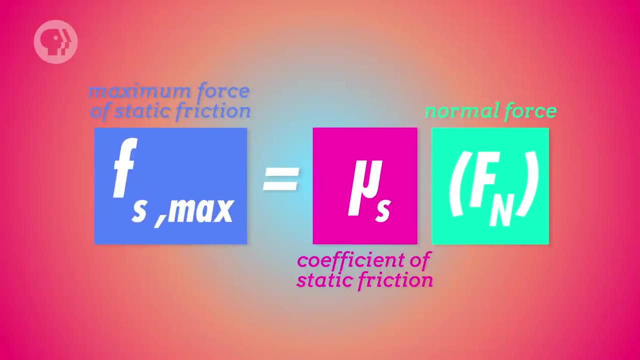 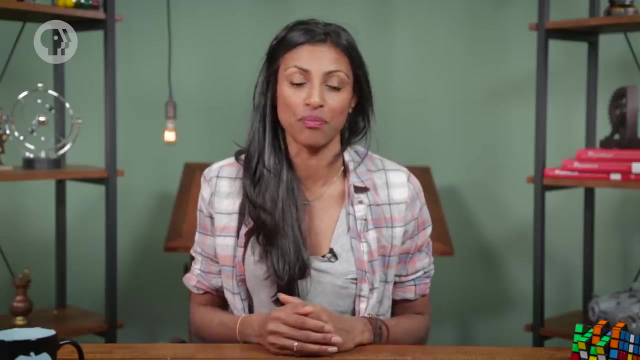 There's even a coefficient of static friction which measures the roughness between any two objects, and we just write it as mus, And the maximum force of static friction is just equal to the coefficient of static friction times the normal force. So now we know the equations for both kinds of friction and where they come from. 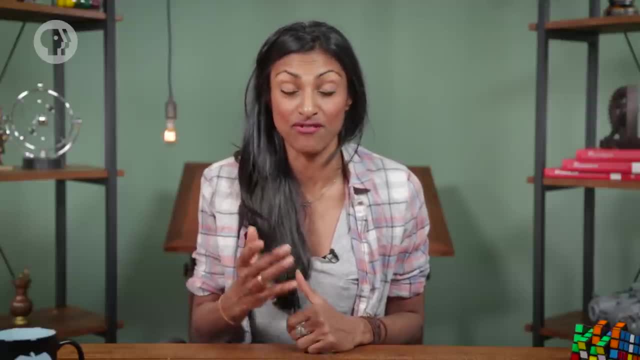 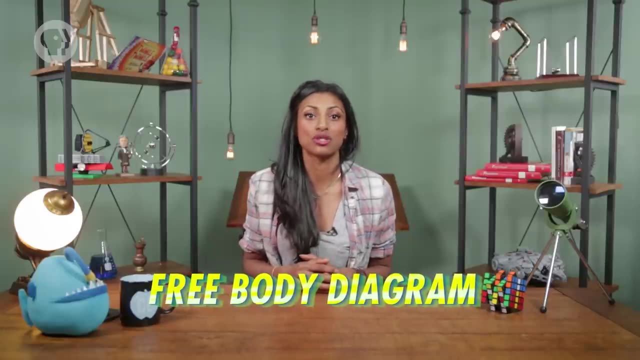 Which means we can use that information to figure out how to solve problems involving friction, Just like with other force-related problems. we start with a free-body diagram That helps sort out what's pushing where, so we can get an overview of the situation. 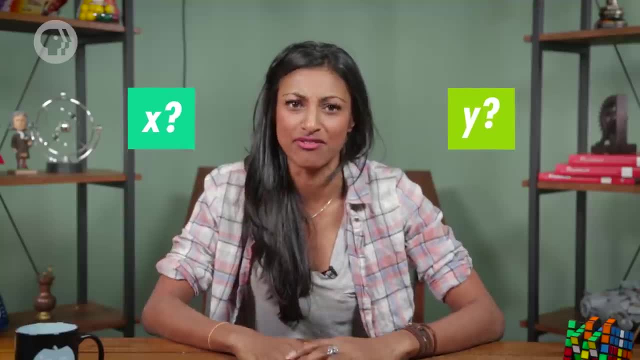 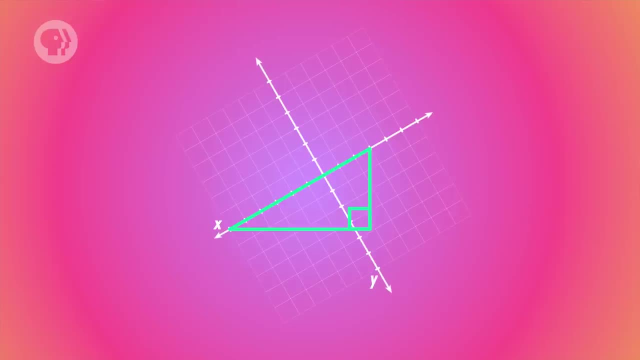 Next we decide on some axes: Where are X and Y and which way is positive. That'll be useful when ramps come up, because, if we want, we can just decide that X points down the ramp and Y points straight into it. 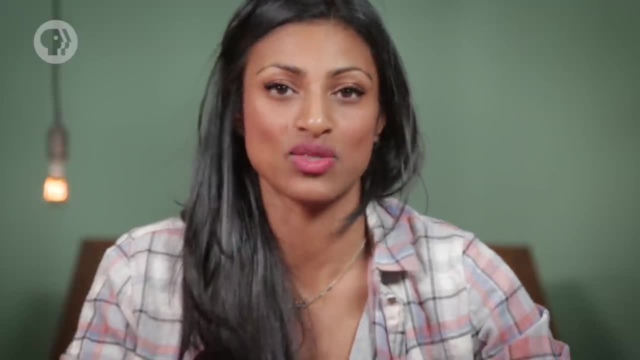 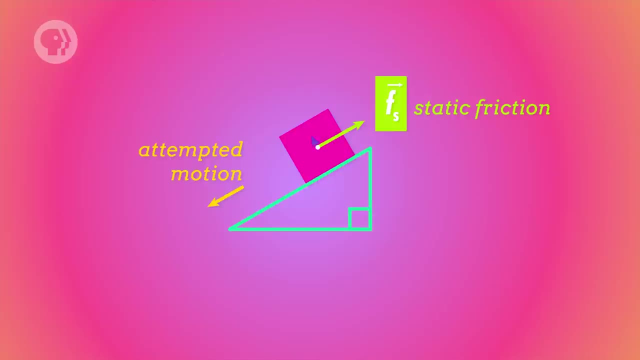 The next thing we'll need to do is separate vectors into components along our new X and Y axis, Because strange things happen to the normal force. when you have something like that bookcase sitting on a ramp, The normal force is pointing out of the ramp because it's perpendicular to the surface. 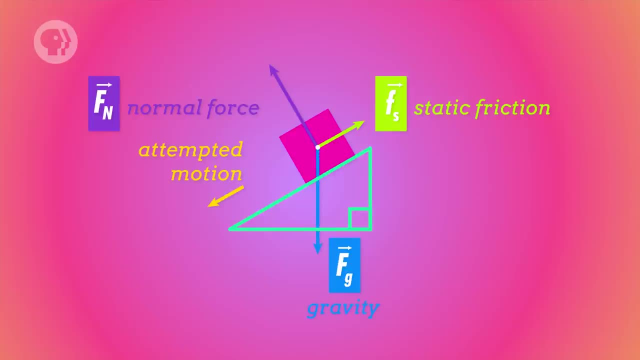 but it's not equal and opposite to the force of gravity, because that's pointing straight down. Instead, we'll have to use trigonometry to separate the force of gravity into two. So we'll have to use trigonometry to separate the force of gravity into two. 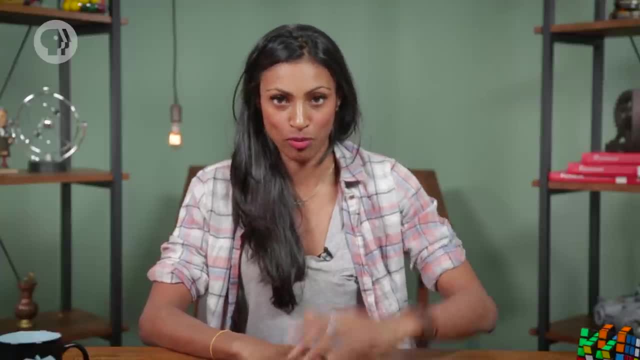 So we'll have to use trigonometry to separate the force of gravity into two. So we'll have to use trigonometry to separate the force of gravity into two perpendicular components, one pointing down along the ramp and one pointing into it. 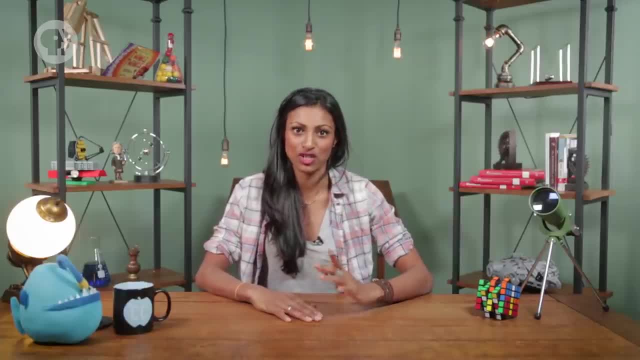 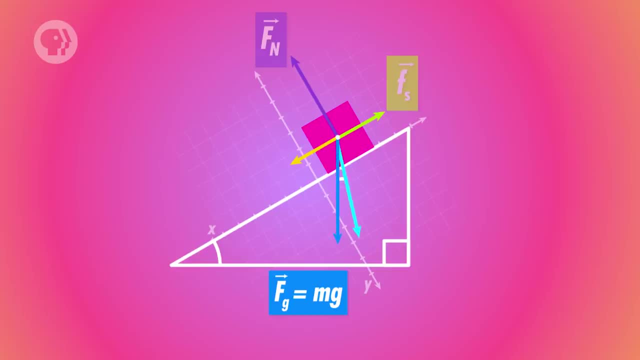 Then the normal force will just be equal and opposite to the part of the gravitational force that's pointing into the ramp. So here's how to separate in diagram everything that's going on. The angle between the force of gravity and the component pointing into the ramp is called. 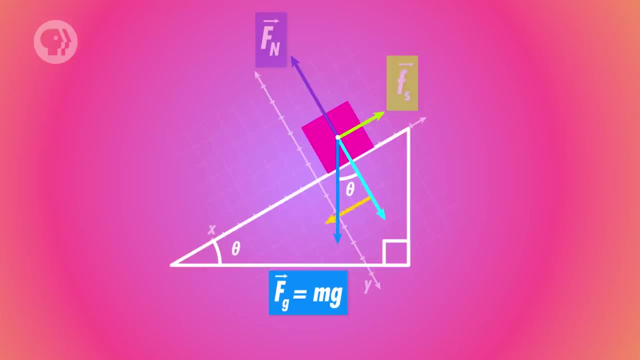 theta and it's the same as the incline of the ramp. Those make two sides of a right-angle triangle And since the component pointing into the ramp is adjacent to the angle, we know that it's equal to mg times the cosine of that angle. 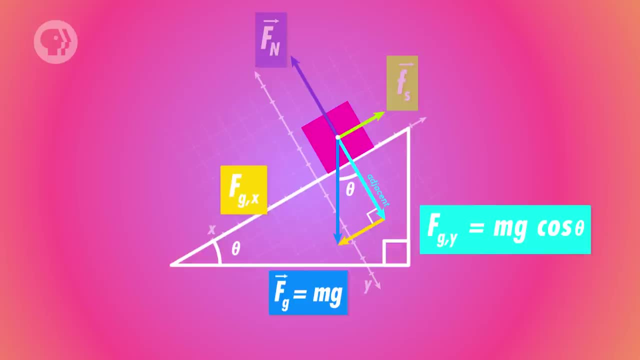 that angle, and so is the normal force. The other component, pointing alongside the ramp, is opposite the angle. So, again using trigonometry, we know that it's equal to mg times the sine of the angle. So you've drawn your free-body diagram, you've decided on axis and separated the 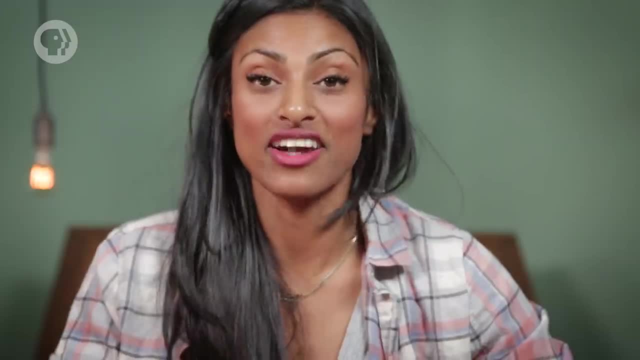 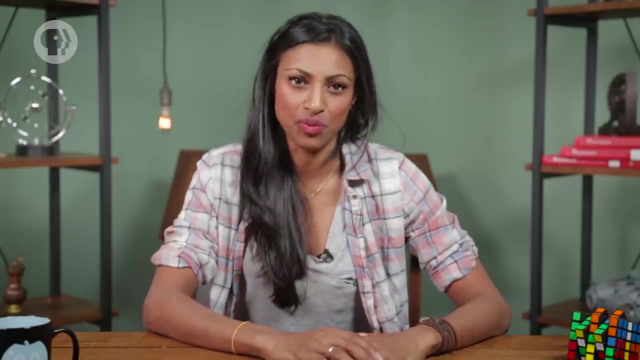 force of gravity into two useful components. Now we can finally set up our equations. That's where Newton's second law, F net equals ma- comes in handy. There'll actually be two of these: one for the x-direction down the ramp and one for 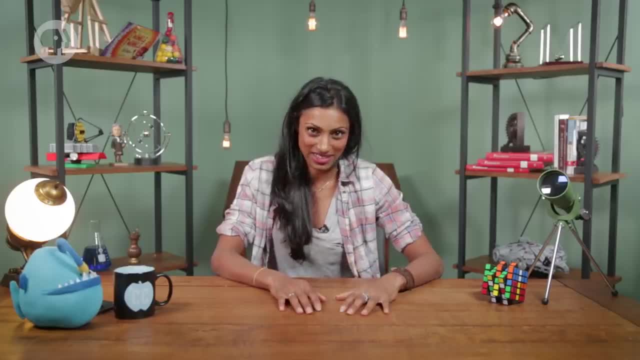 the y-direction into the ramp. So let's say you've got the bookcase where it needs to go and you're ready to get something else out of the moving van, This time a 40-kilogram box with a very fragile vase inside it. 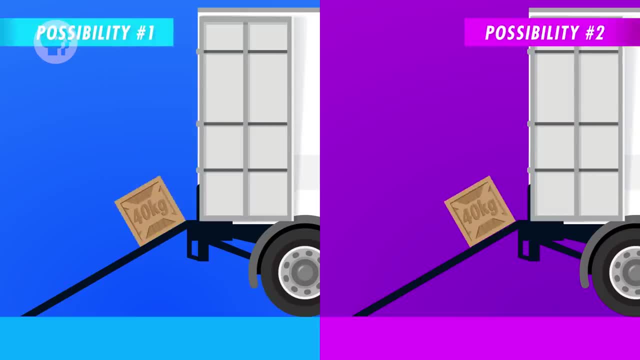 It's heavy. so let's say you put it down on the ramp leading from the back of the truck to the ground, which happens to be angled at 30 degrees, and then you walk away to get a drink of water. You also happen to know that the coefficient of static friction between the box and the 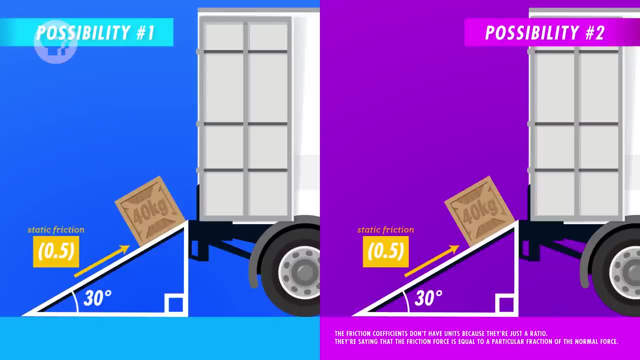 ramp is 0.50.. What is the box's acceleration? If it's zero, it'll stay. Stay put and your vase should be OK when you walk away from it. If not, that means the box will start sliding down the ramp and you may have a problem. 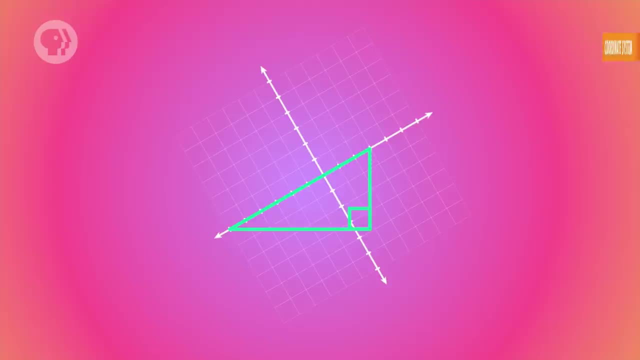 The first thing we need to do is draw a free-body diagram of this box. So the coordinate system will have x along the ramp, with the positive side at the bottom, and y perpendicular to the surface of the ramp, with the positive side also towards. 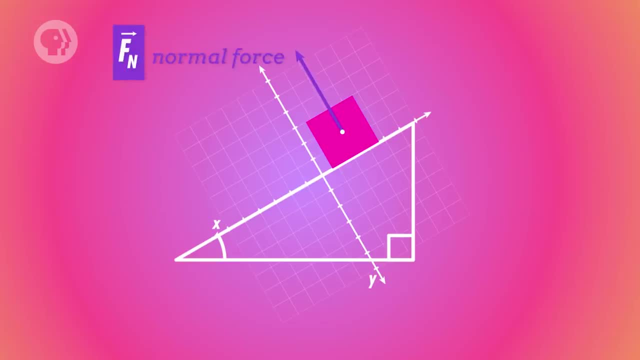 the bottom And we have a whole bunch of forces here. The normal force is pointing out of the ramp. There's also the force of static friction which right now is pointing up the ramp, Since it's resisting the part of the gravitational force pulling the box down. 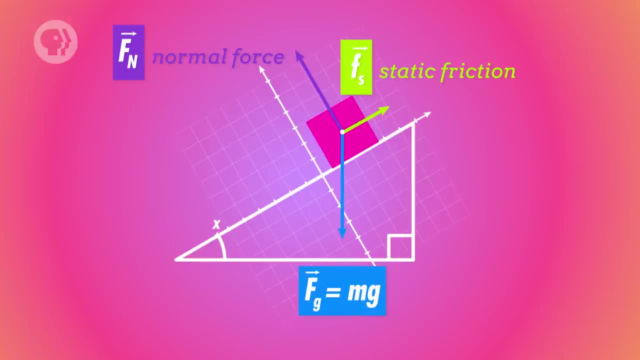 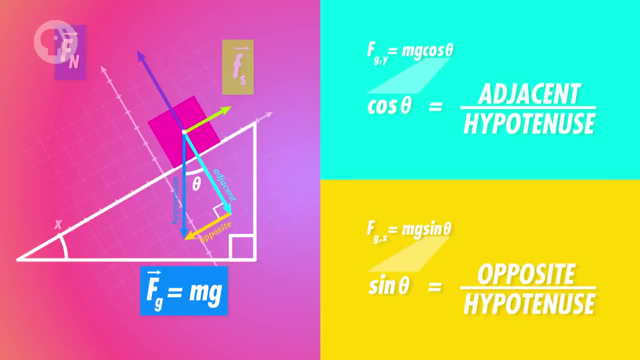 Speaking of which the force of gravity is pointing straight down, not along either of our axes. So we separate it into components: mg cos theta pointing into the ramp, and mg sin theta pointing down along the ramp. Now we set up our net force equations along each axis. 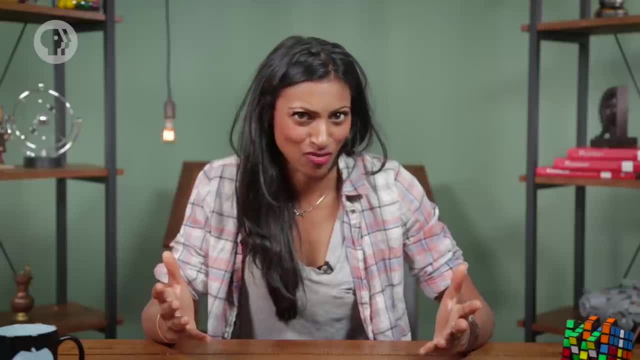 The box isn't going anywhere along the y-axis. Nothing's going to make it start rising above the surface of the ramp right. So we know that all the forces acting along the y-axis should add up to 0.50.. That's right. 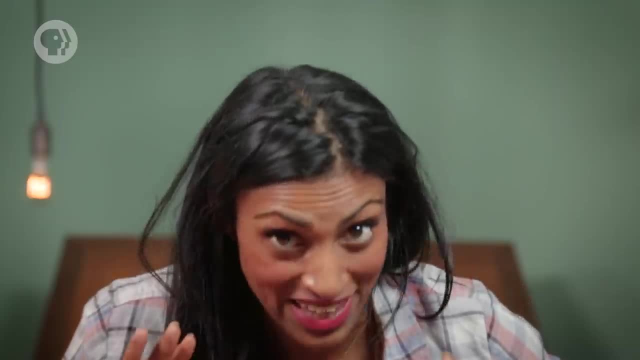 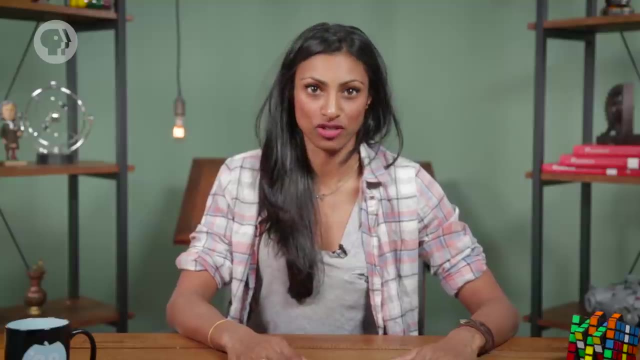 That's right, Since they're all balanced out. But the forces along the x-axis, along the ramp, are a different story. If the box has no acceleration, it's standing still or moving at a constant velocity. They'll also add up to zero. 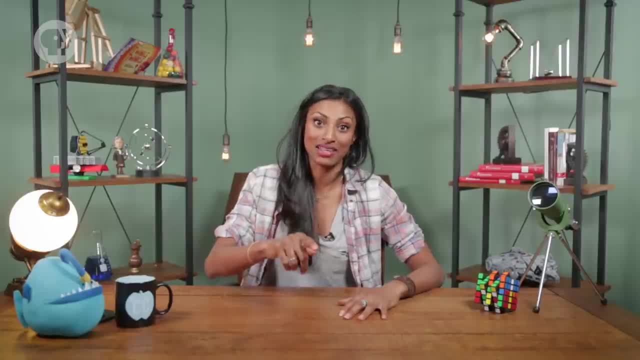 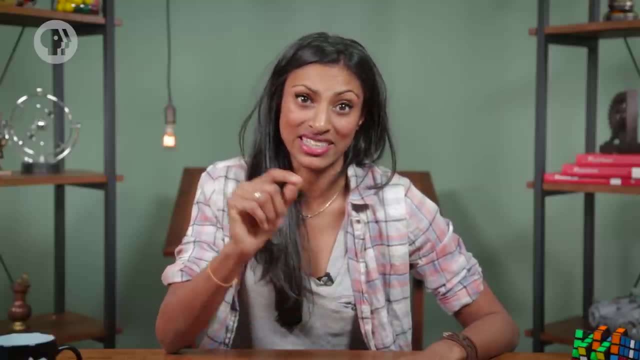 But if it does have acceleration along the ramp, then the forces will add up to its mass times that acceleration. So to figure out if the box slides, all we need to do is find out if the part of the gravitational force pushing it down the ramp, mg, sin, theta, is greater than the maximum. static friction resisting it. In other words, if down the ramp the force is moving at a constant speed, If down the ramp is the positive direction, is the net force positive or zero? The forces here are the gravitational force pushing the box down the ramp. mg sin theta. 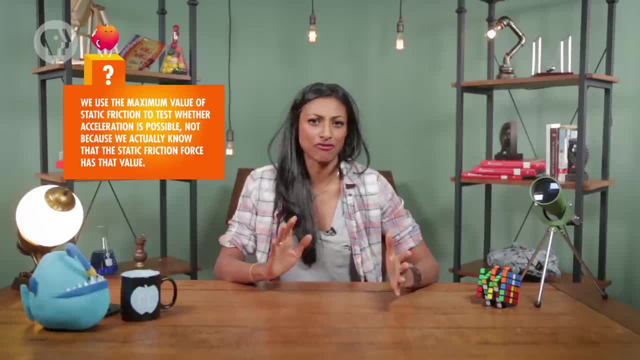 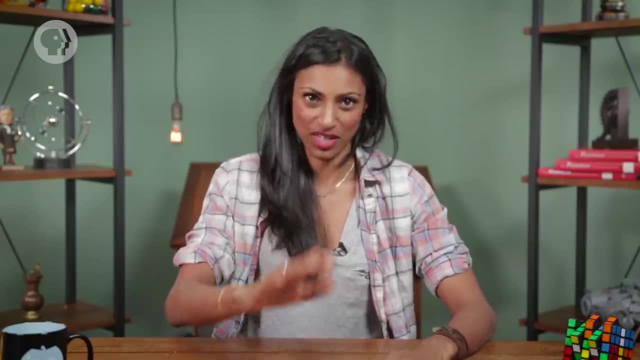 and the maximum static friction. But we write the maximum static friction as negative because it's pointing in the negative direction on our x-axis up the ramp. So adding them together we get this equation. Multiplying together the different values that make up mg, sin, theta, we find that it's 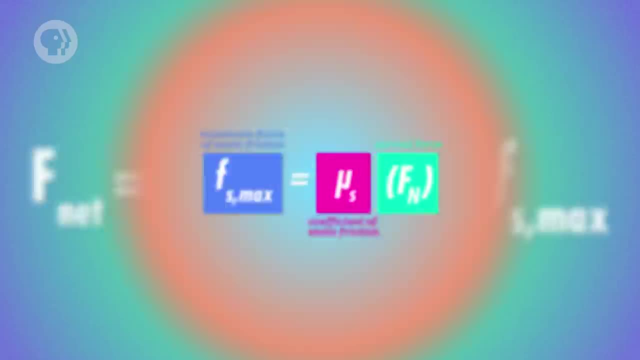 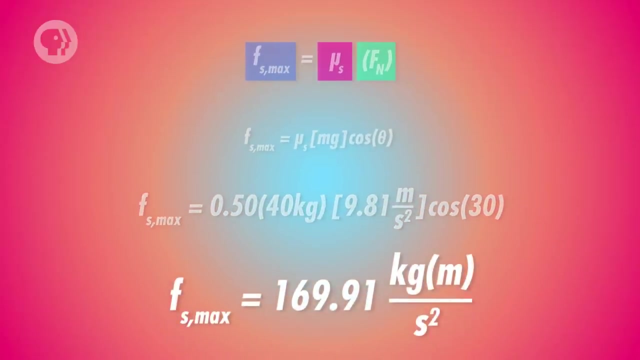 equal to 196.20 Newtons And the maximum static friction is just equal to the maximum static friction. It's just equal to the coefficient of static friction times the normal force. So plugging in the numbers, we find that it's 169.91 Newtons. 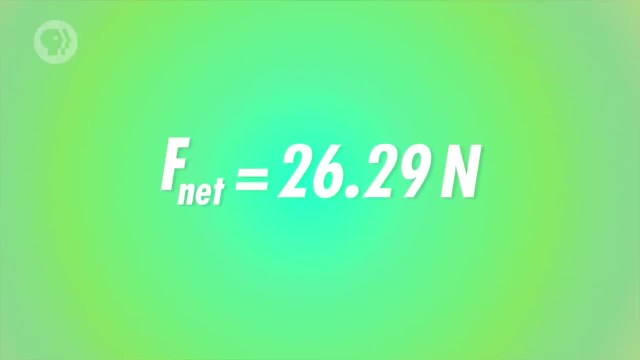 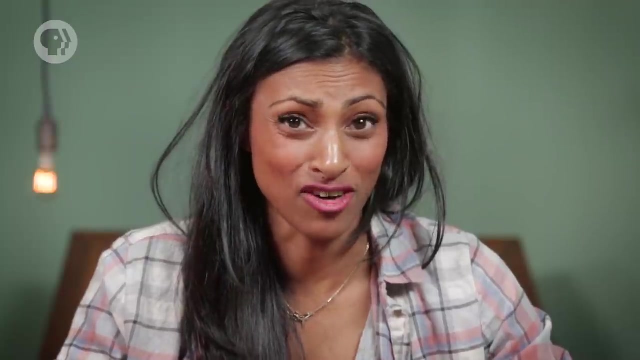 Which means that the net force is 26.29 Newtons. So, yes, there's a net force pushing on the box down the ramp and it's going to slide, Which means I have some bad news for you about that, Vaz. 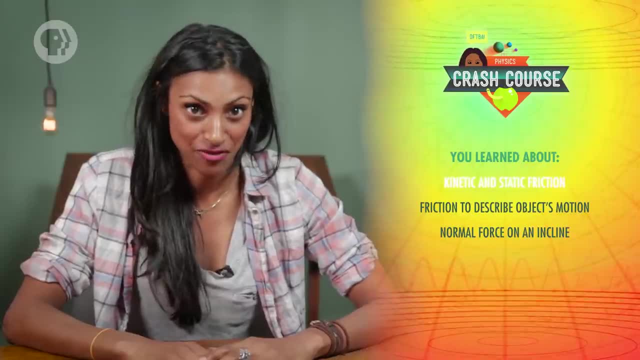 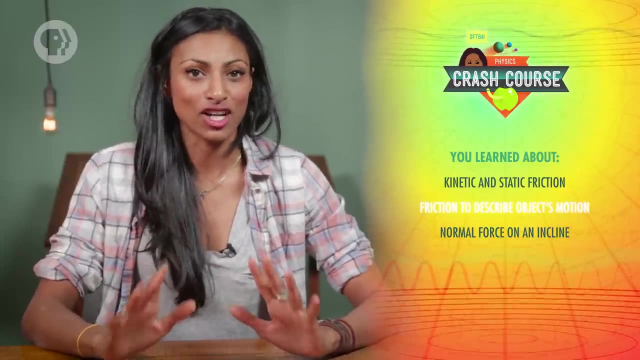 But today you learned about two types of friction- kinetic friction and static friction- and how they act to resist applied forces. We also talked about how to use friction to describe an object's force Motion, including how to calculate the normal force when that object's on a ramp. 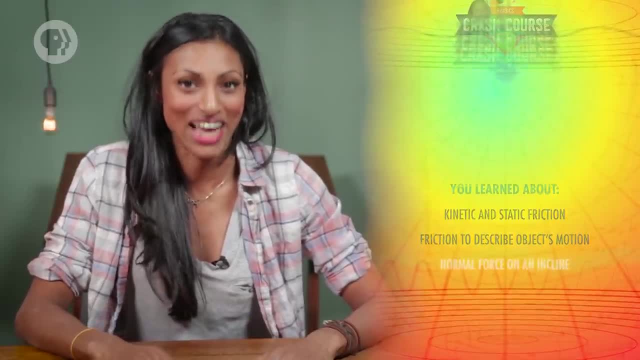 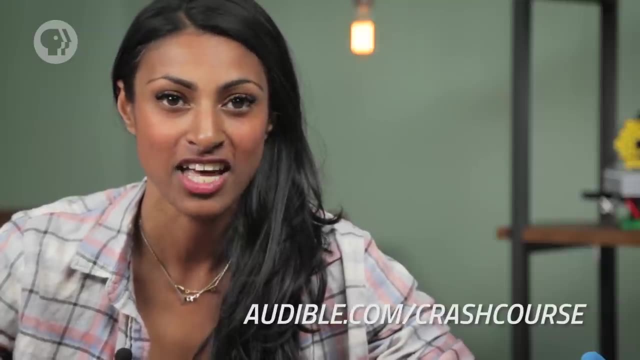 Finally, we calculated whether a box on a ramp would start sliding down. This episode of Crash Course Physics is supported by Audiblecom. Right now, Audible is offering viewers a 30-day trial period. Just go to audiblecom. slash crash course. 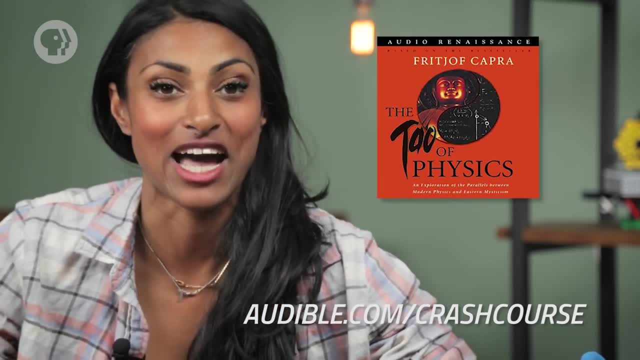 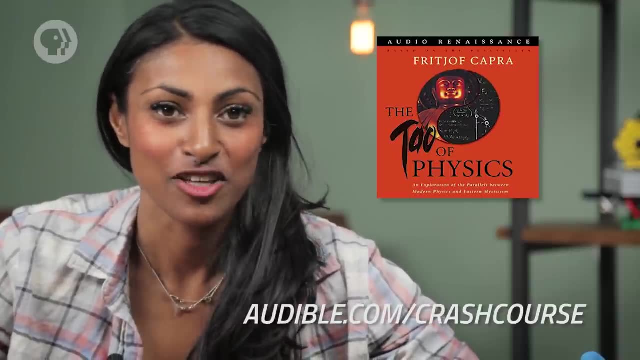 You can access their audio programs and titles like this book, The Tower of Physics by Fritjof Capra. My plan is to listen to this on my flight back home this week. It's a long flight. Go to audiblecom. slash crash course. 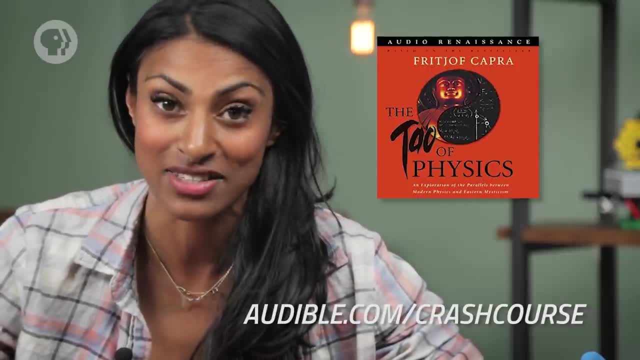 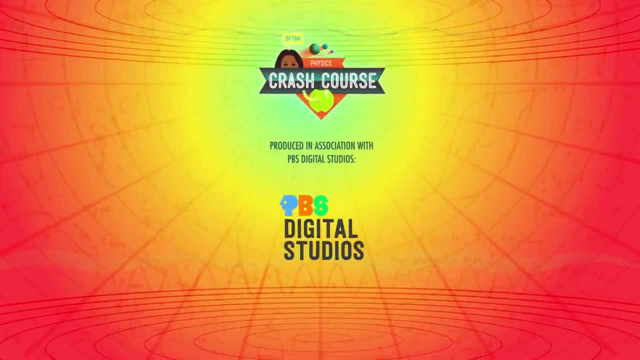 And make sure you use that link to help us out and to get your membership trial. Crash Course Physics is produced in association with PBS Digital Studios. You can head over to their channel to check out amazing shows like Deep Look, The Good Stuff and PBS Space Time. 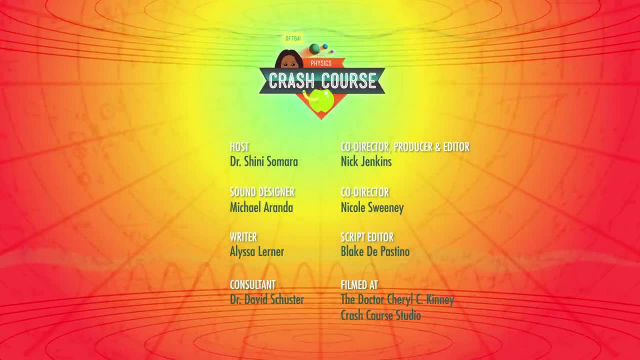 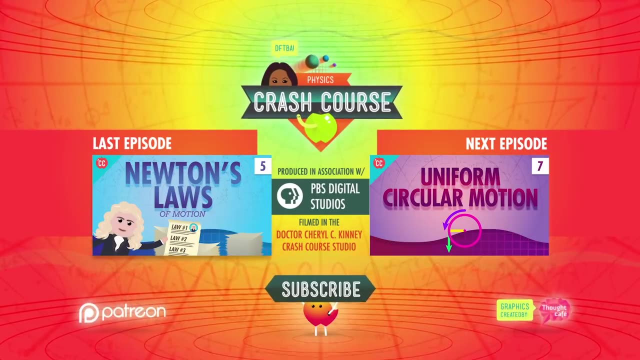 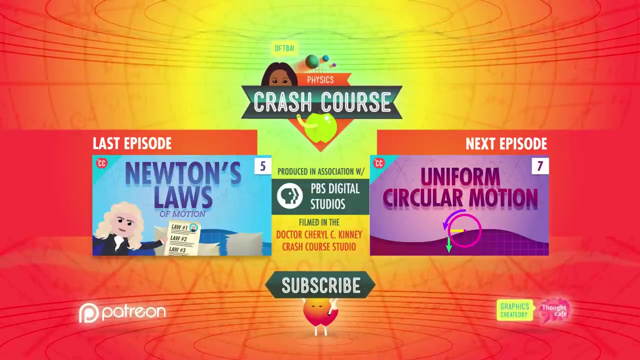 This episode of Crash Course was filmed in the Dr Cheryl C Kinney Crash Course Studio With the help of these amazing people, and our graphics team is Thought Cafe. Thanks for watching. We'll see you next time. Bye, Bye, Bye. 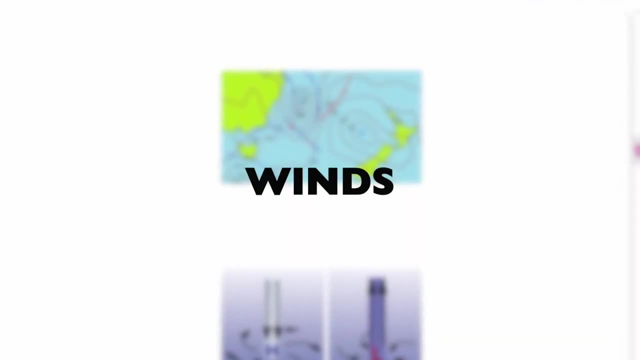 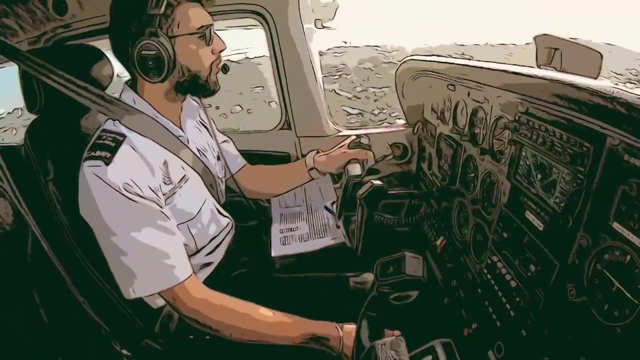 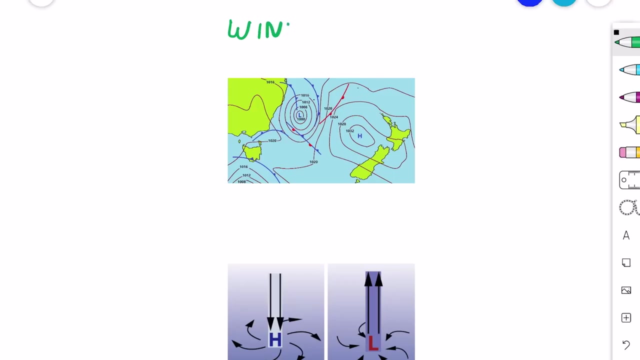 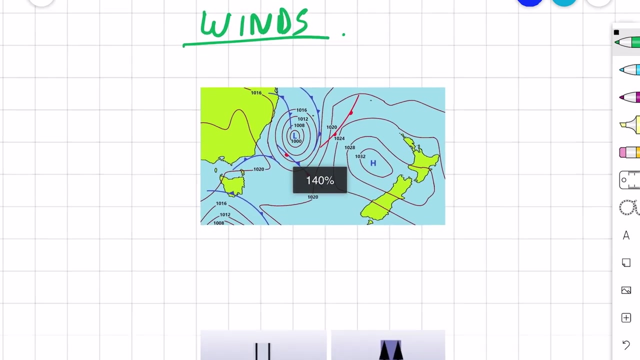 Hello everyone. so I've received a lot of requests for a video on winds. Here it is and I hope it helps you. Before talking about winds, let's talk a bit about surface pressure. So the surface pressure of any location is plotted on a surface pressure chart. 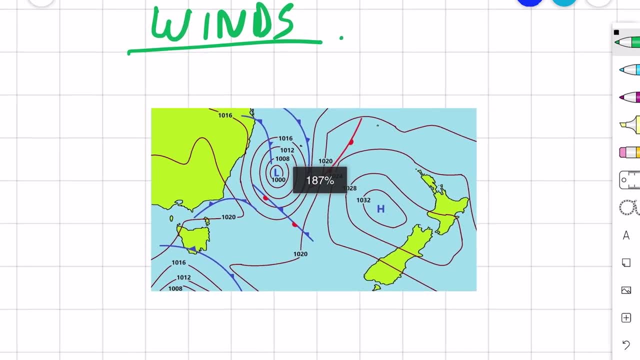 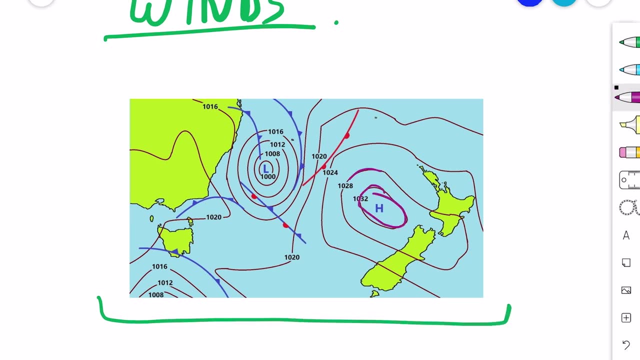 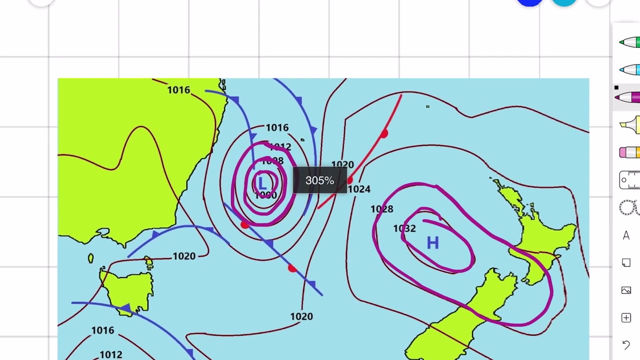 These charts have lines of equal pressure known as isobars. So this is a surface pressure chart and the lines you see in this, these are the isobars. So isobars are the lines joining places of equal pressure. So, for example, on this 1016, the pressure throughout the isobar will be 1016.. 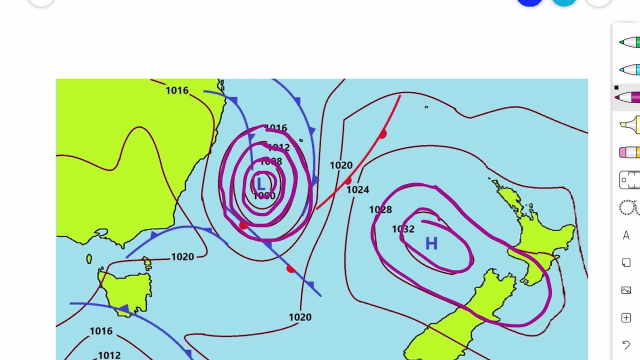 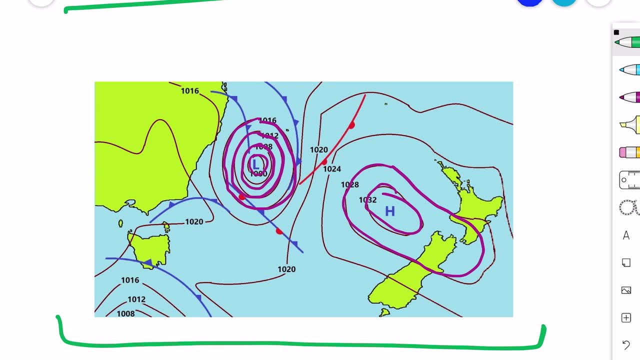 In fact it's joining all the places where the pressure is 1016.. So these are known as isobars, and each isobar will have a number written on it which will represent the pressure of the isobar. So, for example, this is 1024.. 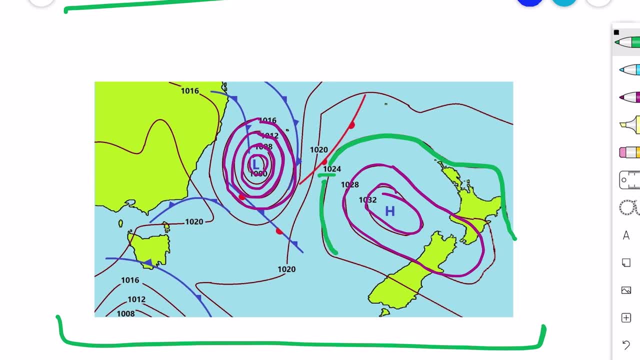 That means that on this isobar the pressure is 1024 hectopascals Right Now. these isobars explain a lot about wind speeds, So the closeness between two isobars will give us an idea about the wind speed. 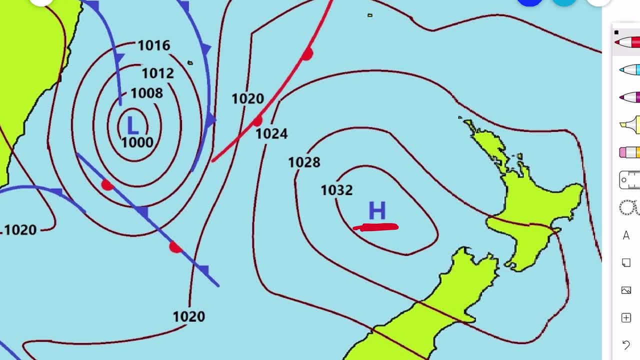 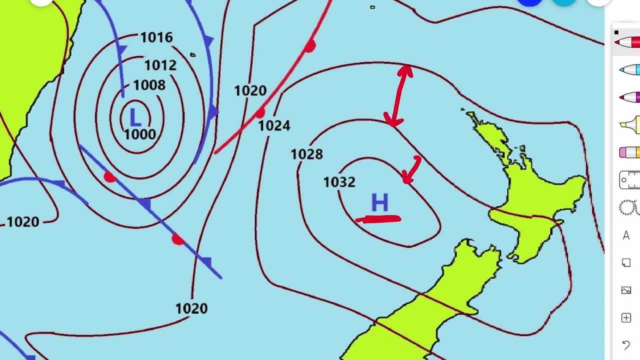 Like, if we see around this, H H stands for a high pressure area. So in a high pressure area, if we see the distance between two isobars, it's a lot Over here as well. And now if you compare this distance to a low pressure area, which is over here,